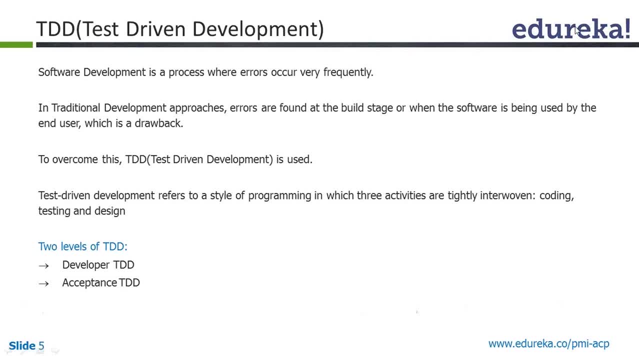 So test driven development is nothing but where your code is driven from your test cases. So whenever you have a requirement in Agile, whenever you write a requirement, you draw acceptance criteria against it. When you are doing the discussion, when you are having a conversation with your product owner and with the complete team involvement. So when 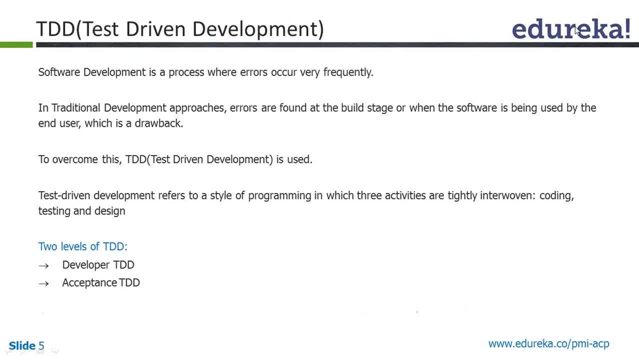 you have your acceptance test cases. having those test cases in mind, you create your code. So under this there are two ways of doing it. So the first way is to create a code. One is acceptance test driven TDD and another is developer TDD. So in the developer. 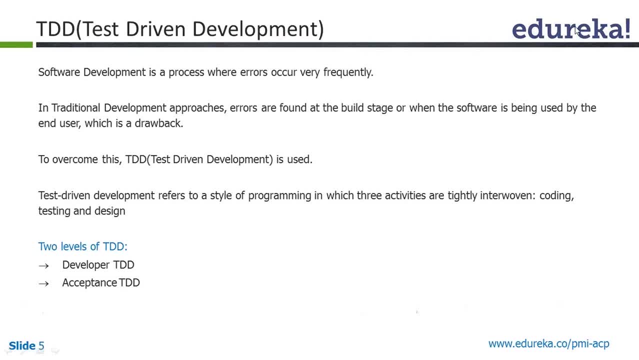 TDD, the test scenarios that you are creating out of the acceptance criteria would be written by a developer, So you would be creating your code from a unit test case, in a way, While in ATD you would be a tester would be creating the test scenarios out from the acceptance. 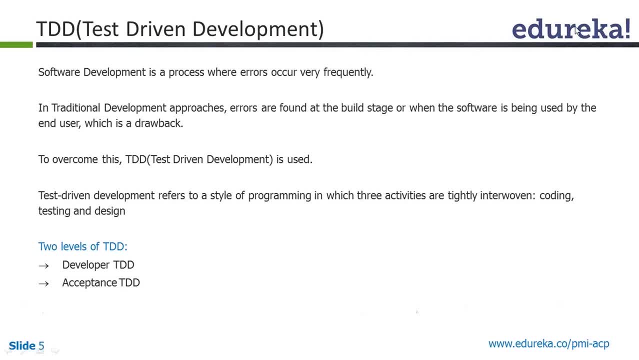 criteria and from those test scenarios you would be creating the your code. So you would be creating your code out of it. So the only difference is from that is that ATD would be obviously more detailed, because obviously a tester would have more detailed scenarios. 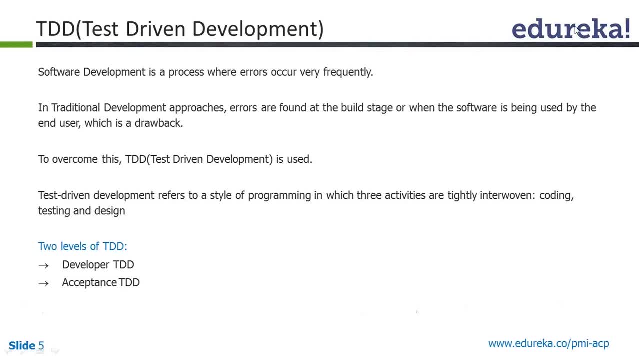 like he would. he or she would think about all the negative, positive and all the boundary value values, Right, While a developer would not get into those left details. So ATD is obviously more detailed. So I'll give you, I'll, we will, I'll just showcase you flow. 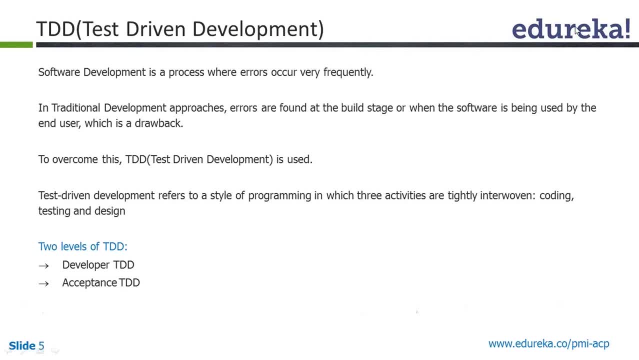 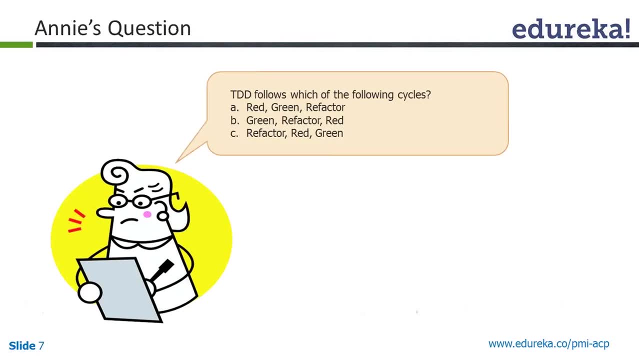 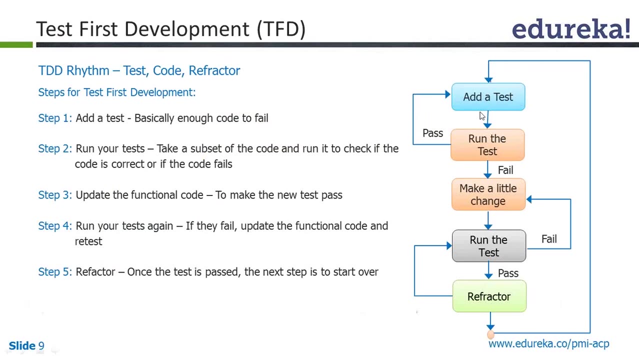 chart which will help you understand more about it. Okay, So, before we talk about this stage, let me show you one. this: Okay, So what? what we say is you create a test which is called add a test. Okay, Test case. Then you 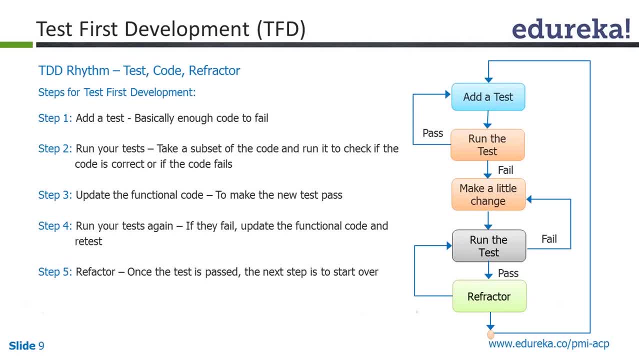 run that test case even before your development has happened. Okay, So you have a story. you you create a story, a acceptance criteria when you started discussing it with the product owner- correct. Now, from that acceptance criteria, you start writing your test scenarios based on those. 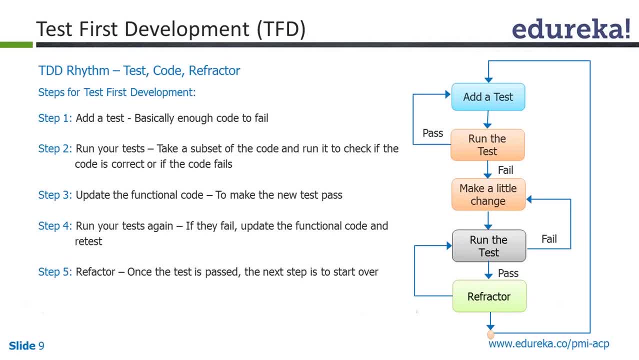 testing criteria, acceptance criteria. Now, once your test scenarios are complete, you run it For the first time, very first time. it will fail, correct, Because there is no code written against those test cases. It will fail Now, for example, if I have to create a login screen. I got all the acceptance criteria. 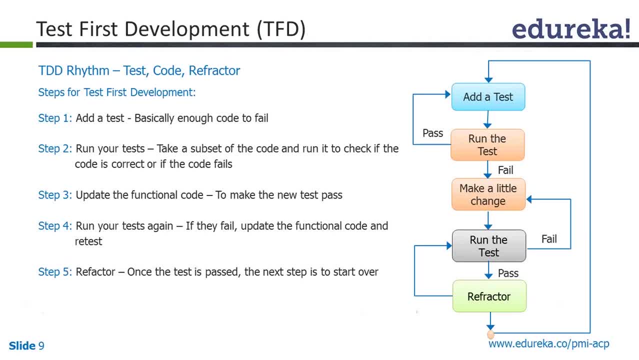 I ran my all the test cases. It will fail because there is no login screen implementation. that has happened. Now, once my test scenarios are in place, Looking at those test scenarios, my development team will start making a developing a code out of it. okay. 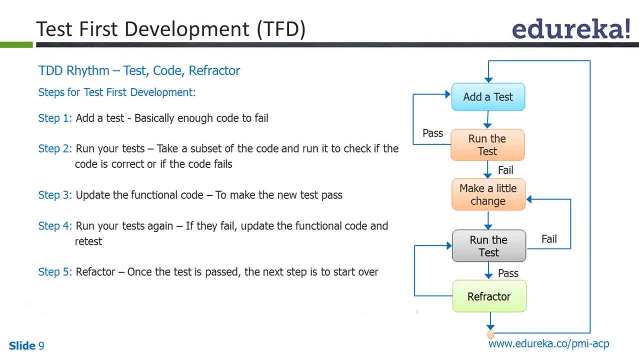 So my, for example, if my first test scenario says it should have a user name text field and it should have a password text field and a submit button, I'll just add those three. Even if my first test scenario doesn't talk about labels, I will not add it. 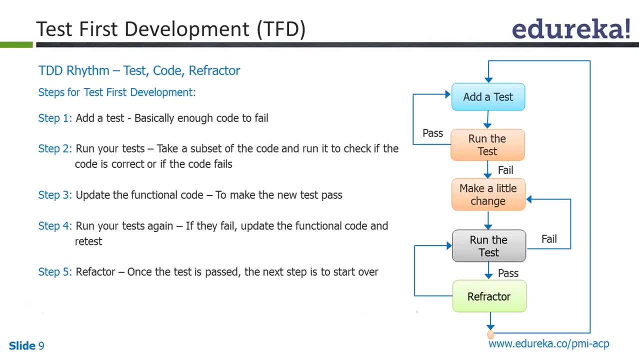 The test would. The second would say it should be: it should accept more than four characters in the user name field and the password should not take any special characters. So my testing, my code, would be written against it. I would not implement anything extra fine. 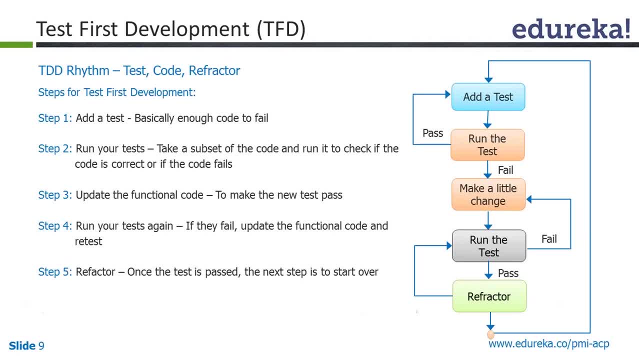 Now, once I have done all the coding against my test scenarios, I'll again run it. In this case, some of them would pass and some of them would fail. There could. there is a possibility that everyone- everything- would pass If my test developer was smart enough. correct, right? 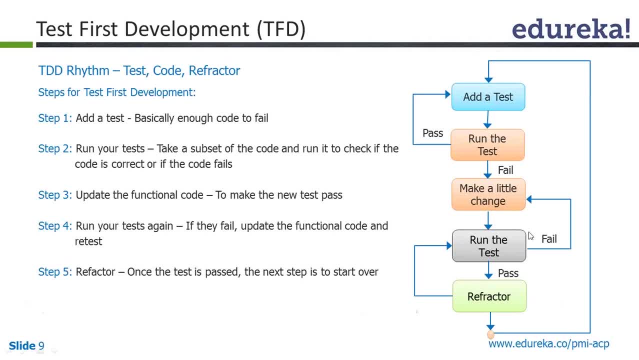 Now, when I do this this second time, when I run it, if it passes, I would refactor my code. When I say I would refactor my code, I would go back and make all the you know coding. I would make the changes according to the coding standards because, obviously, since 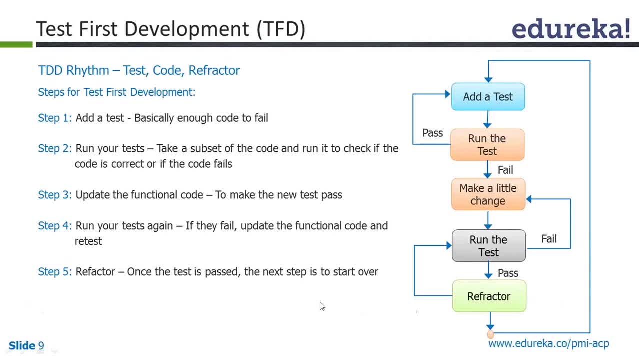 I was running it through, I would, I would, I would have written dirty code, I would not have, you know, made any proper, you know proper variables and I would not have added any labels across it. I was just testing what my, I was just making what my test case recommended. 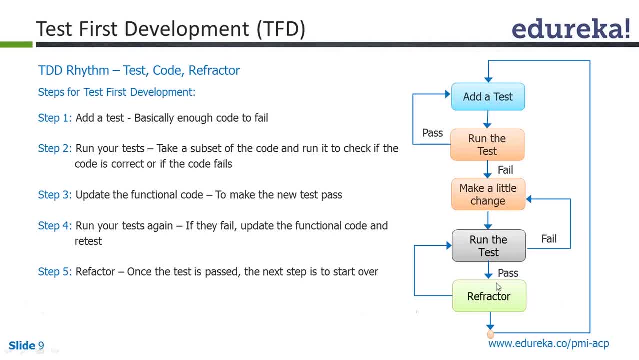 Once my refactoring is done, I would again run and would, if it passes. if it needs further refactoring, I would do it. Otherwise I'll stop it there And would move to the next, To the next requirement. If it fails, I'll keep on changing my code till the time my my complete test set passes. 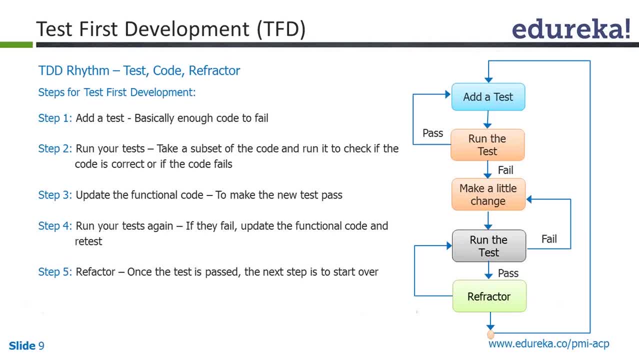 Okay, Yeah, Is it making sense? Yeah, it's clear. Right, Though the only benefit of having this, this is because you are picking up the code. you are making the changes at a very smaller level. You are not making bulk changes. 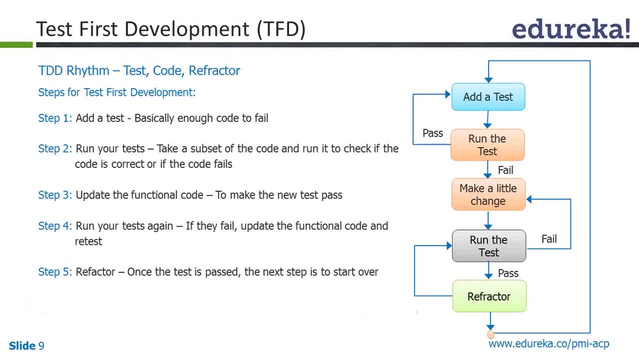 You are not doing a big bang work over it. You are making changes at a very small level, You know, picking up small set of requirements. you are making the changes. So whenever. if you are making a change right, you would know what: five lines or ten lines. 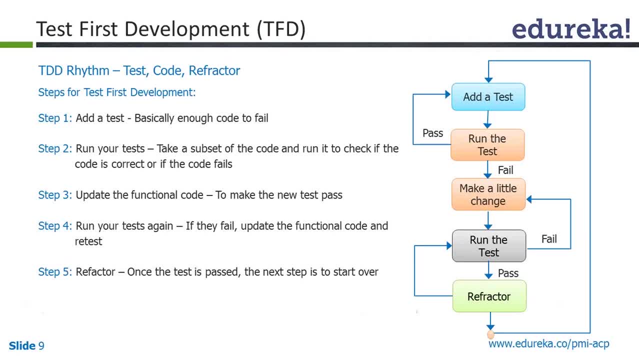 I changed. So if there is a problem after a small change, you would. you would know only these ten lines would have a problem, because when I just wrote a basic code, my things were working. Now, while I was imperfecting it, I was adding more things to it. it it bonked down. 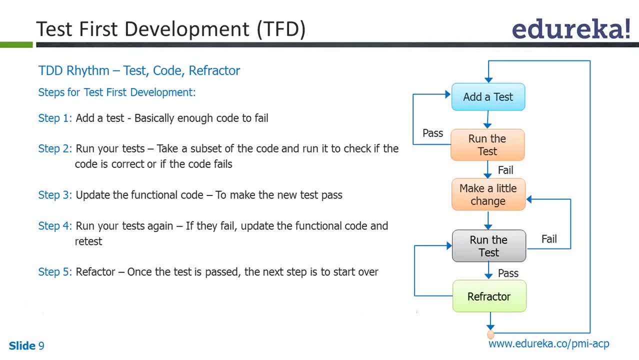 Right. So it will help me and it it will help me judge the problem correctly. It would help me understand the problem area: what, which, which? which is wrong? Now looking at this diagram. this diagram can be divided into two sections. 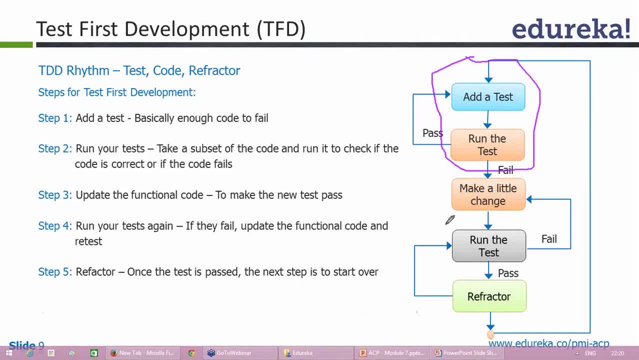 One is this, Another is this, This, This, And third is this. Now, this first section is called red. Why is it called red? Because everything is failing here. I just wrote the test cases. no, then there was nothing which was coded, so it would fail. 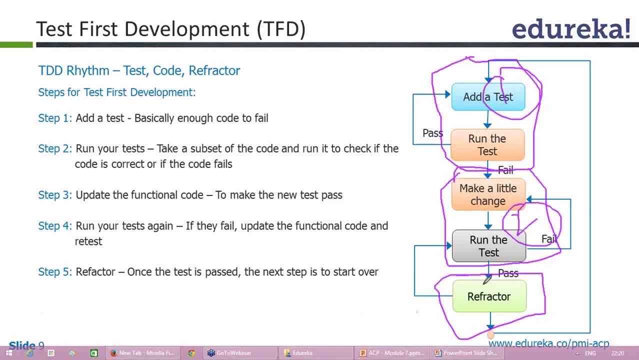 Second is this: This is called green, Red, green. And third is refactor. This is called green because I made, I wrote a code And I was executing it, So something is passing and something is failing, or everything could pass Right. 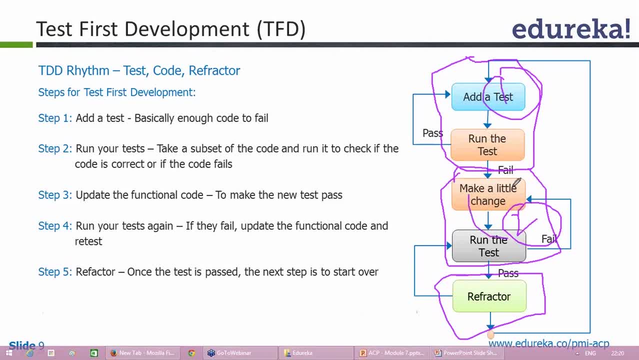 I would only move out of this green when everything passes. I would not come to a refactor stage till the time whatever I implemented or whatever code I developed is not has not passed. I would not come to the refactor stage. I will keep on coding till my first set of things were are not green. 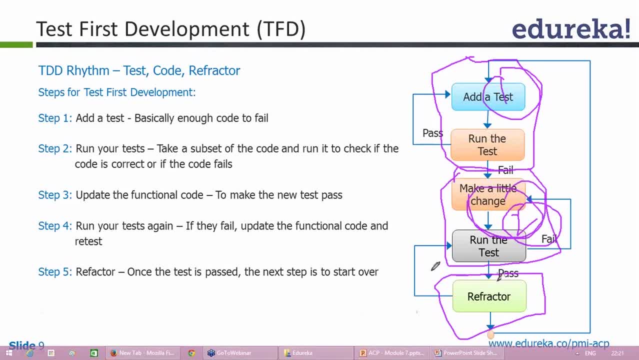 I have not executed. I have not executed properly. Okay, Red green refactor. Okay, So this is what we were discussing, Okay, So this is what I was wanting you to tell you. So, in TDD, TDD follows red green refactor. 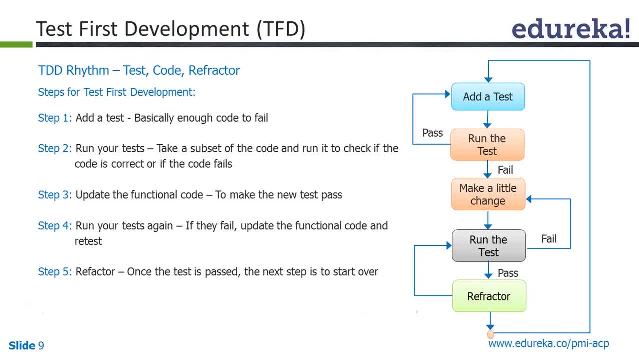 Okay, So this is red green refactor cycle. Clear Red is writing and filling the automated testing before writing the production code. Green is making a minimal change to production code to fix the failing test. So I will not come out of that production code, of that code, till it passes. 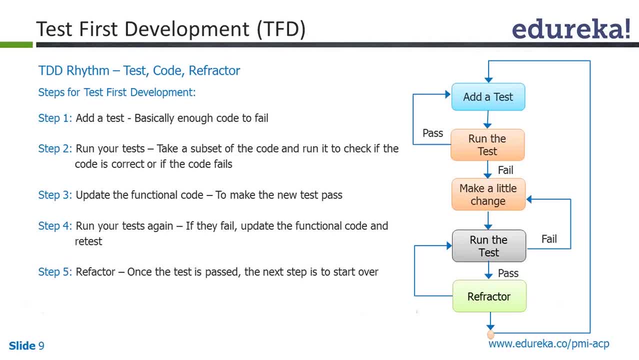 Hence it is green. The third is refactor, where I am improvising my code. I have written all the enough test cases. I have written enough code to pass the the test, Okay, Okay. So I have written that particular, that particular test case. 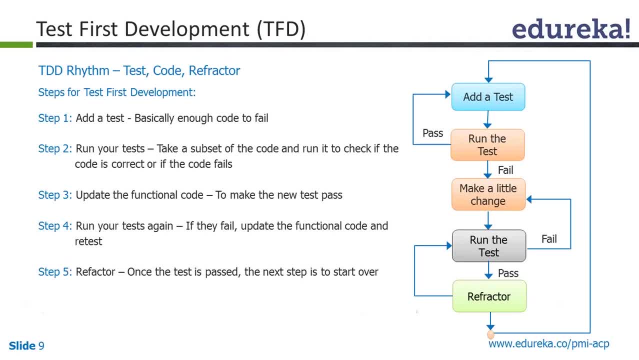 Now I would go back and make it, improve it. I would make sure that there are no duplicate variables being used. It is readable enough. I will start. probably I will go ahead and add the comment to it. I will make try to make it simple. 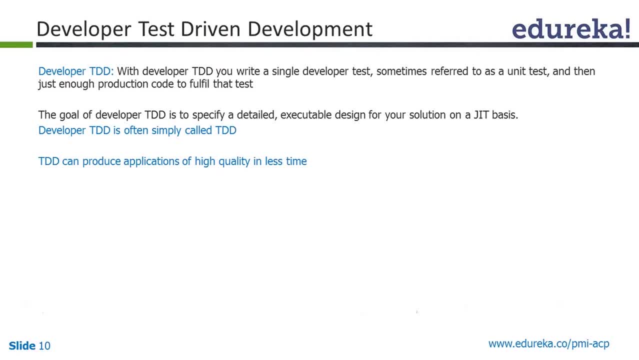 Okay. So, as I told you, DDTD, developer-driven development, so it is something with the developer. You write a single developer test, sometimes referred to as a unit test, And then just enough production code to fulfill that test. So the goal of the developer DDTD is just to specify a detailed and executable design. 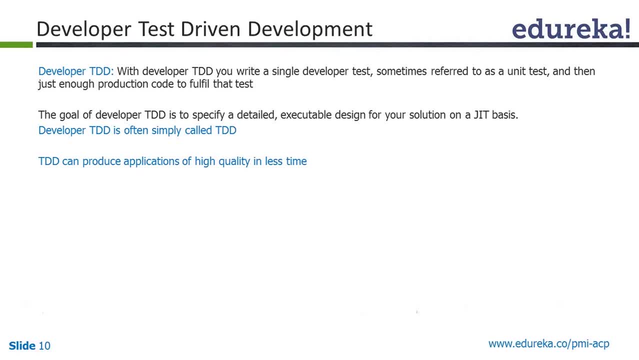 So you are doing something which is just needed to pass the test. You are not thinking that all the positive and negative scenarios you are doing which is just needed, the minimal thing you are doing. You have not thought of any negative scenario. So, for example, if my password 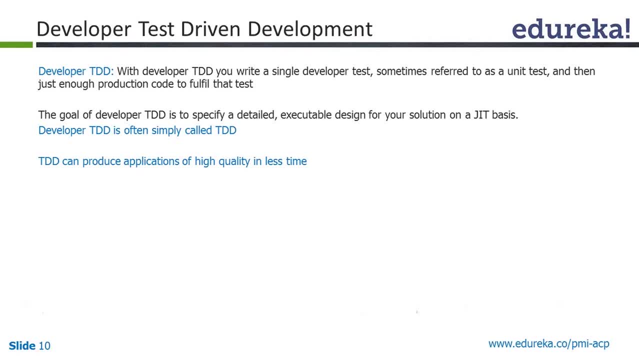 Okay, I accept from 8 to 20 characters, right? I did not write a code which said that what will happen if I entered 7 characters to it? It will not. it will not think of that level, right? So you are just writing a minimum basic thing that will just pass your test, okay. 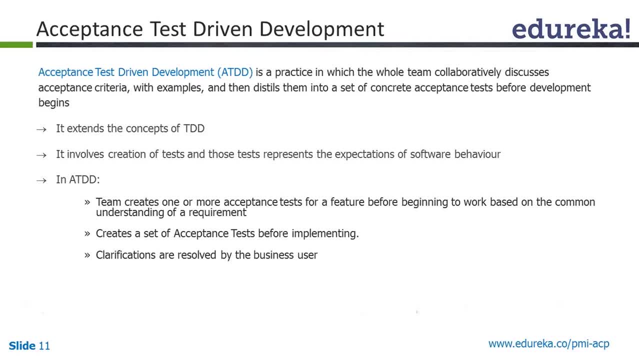 And acceptance again is a Okay. It is a practice in which the whole team collaboratively discusses the acceptance criteria. They have the complete acceptance listed with them and they detail it out to as much level as much possible. Okay, So acceptance test criteria is obviously a more detailed information, because you are 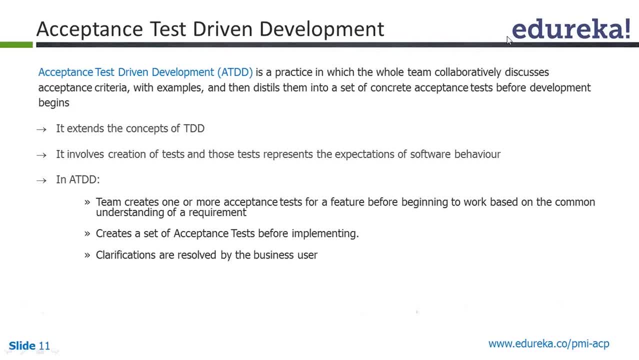 detailing it with your product owner. This is as simple as right. Somebody doing a Unit testing. even if your teams are falling in the unit testing, you still find defects in your functional testing. So there are two terms which are used for implementing TDD. 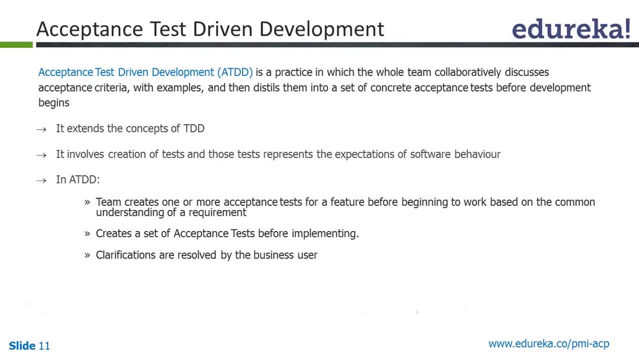 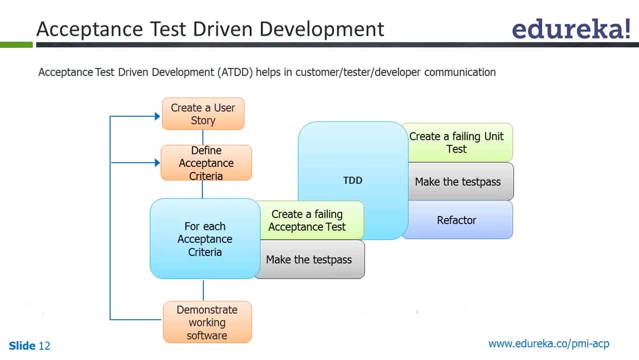 One is KISS, This is, keep it short and simple. Another is YAGNI, YAGNI. I will just spell it for you, Okay? So I think this will again help you Acceptance. test-driven development helps in customer. 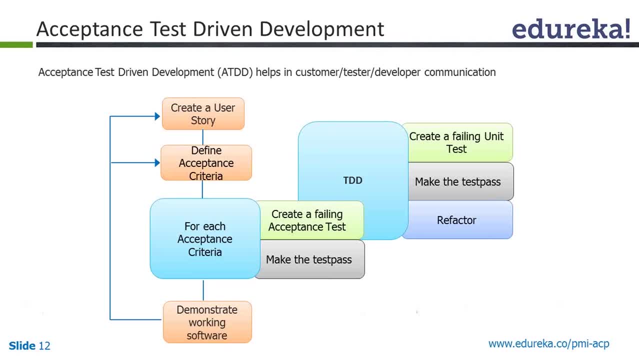 You are. so this is a flow chart. So what is happening? You are creating a user story. You are defining acceptance criteria. For each acceptance criteria, we are defining both the positive and negative scenarios- This one. Right Now I am passing the test cases. 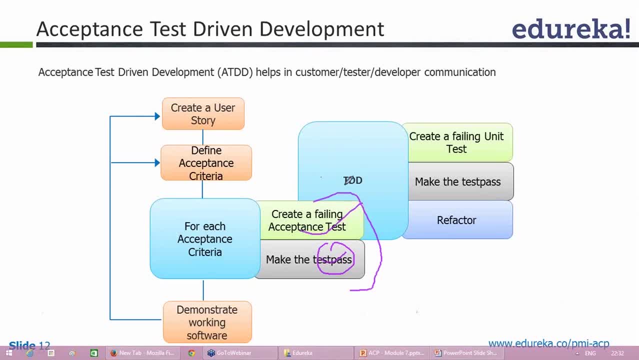 Right. This is where my TDD is coming. For each acceptance criteria I have both positive and negative, And I am making my test cases pass through it. I am refactoring my code And, once this is done, I am demonstrating my work software. 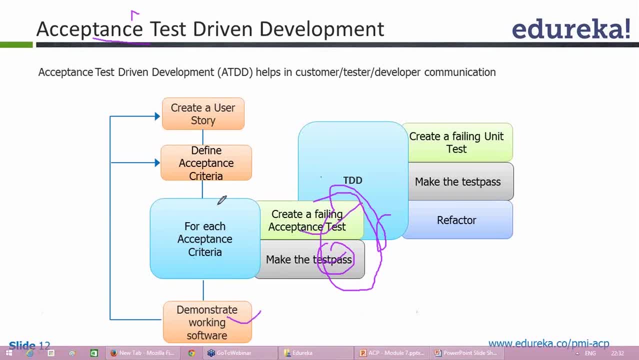 While in developer, test-driven development, for each acceptance criteria, I would just have my unit test cases. It would not be against each. No, Because my acceptance criteria are defined. I would just have unit test cases. I would not have a detailed test case plans for each scenario. 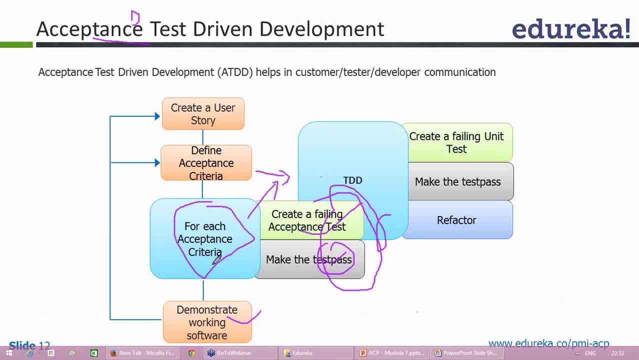 It could be on a very high level. Got it Plus. in this case, my product owner is involved at each stage. When I am writing acceptance test scenarios, I am involving my product owner at each stage. Okay, I am assuming my product owner as well. 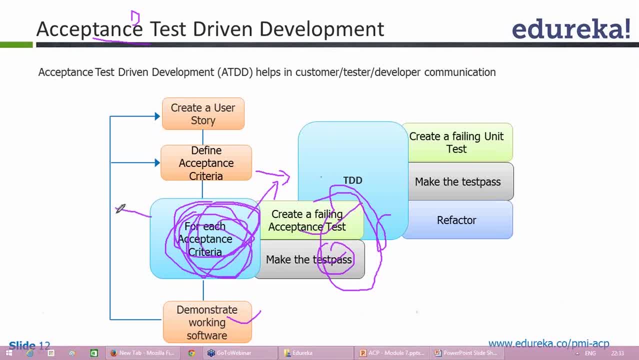 But in developer-driven test cases, my product owner is not. This is done by my dev team. Okay, And my test cases where my product owner is being involved is the functional testing where they are getting involved. My detailed level of scenarios are being created for the functional test cases. 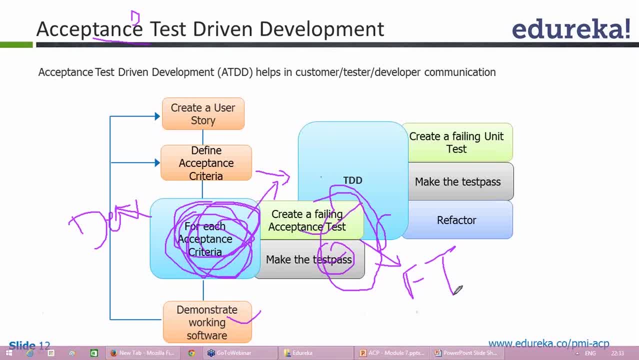 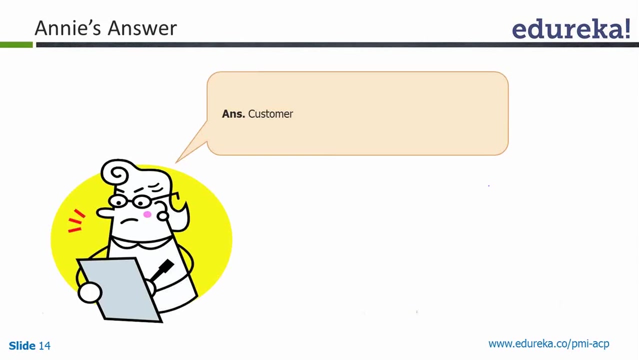 Okay, Got it. Yeah, Yeah, Madhuri, is that clear? Okay, Yeah, So I was mentioning about to achieve test-driven development. there are two techniques that we use. First is called Keep It Short and Simple, That is KISS. that is the acronym KISS, and another one is YAGNI. 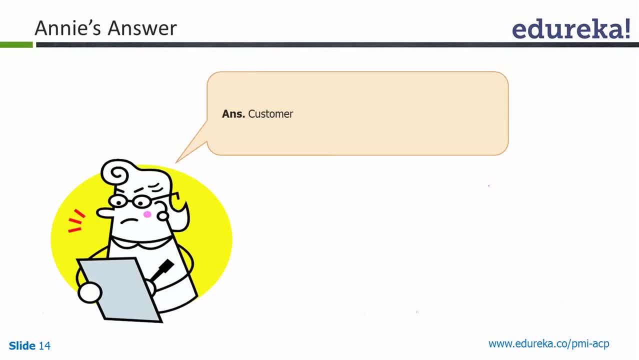 YAGNI is: You Are Not Gonna Need It, Y-A-G-N-I. So this comes from a factor that in Agile we are deferring the decisions as late as possible, and we are so in NTDD we are coding only something. that is much that the minimum. 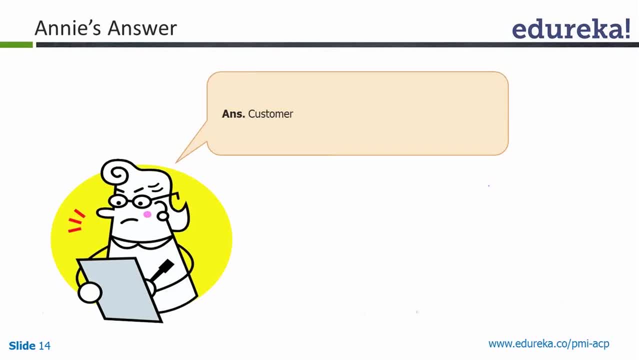 amount of something that is needed. We are not elaborating it. we are not going beyond what is not written in a test case first, Like, if my test cases doesn't talk about labels, I am not adding it. okay, So two terms that you need to remember is KISS, YAGNI. 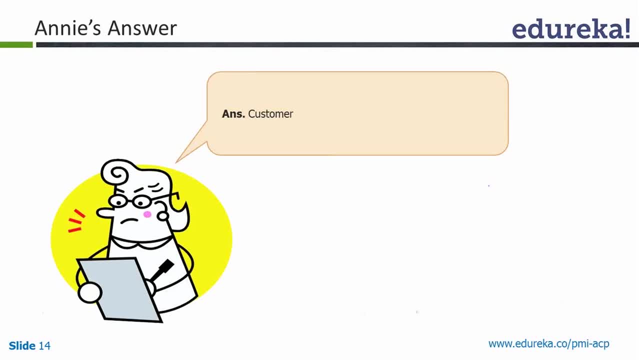 Okay, who specifies acceptance tests in an Agile project Testers? Uh-huh, Customer. product owner: Okay, Product owner is the right answer, not the customer is not the correct word here. product owner, Product, You remember? 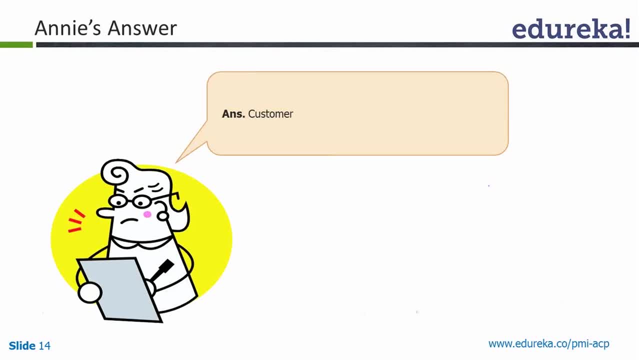 Product owner is the one who, even when you were doing your planning poker- you were, you know. Product owner was the one who was clearing all your doubts. he was giving answers to your assumptions. he was clarifying: do you need a yearly pass? monthly pass, what would? 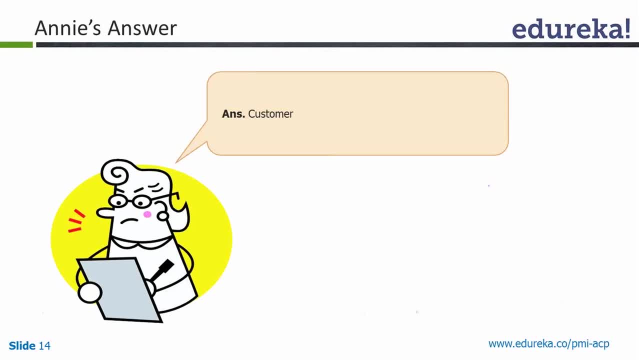 be the renewal process. he was the one who was giving all the clarification. He is the one who specifies the documentation can be done by anyone, but it's the product owner who defines the acceptance criteria. Absolutely Correct, Okay, The technique in which participants collaboratively discuss acceptance criteria and distill them. 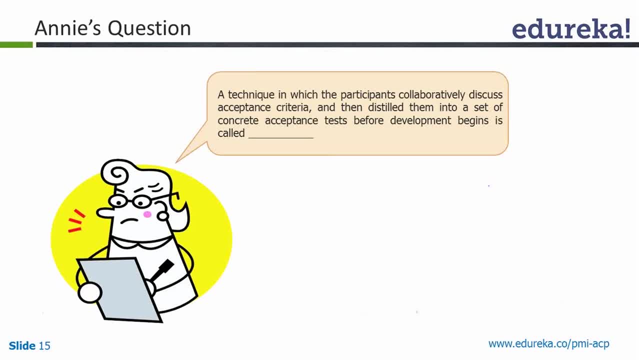 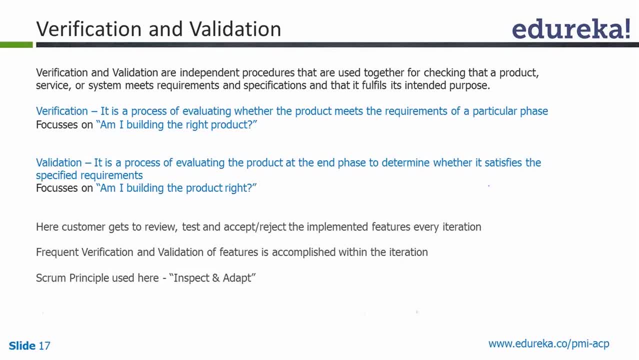 Okay, Okay. So let's come to a basic testing, and this is what you are going to teach me now, Can you? so what is verification and validation? first thing, Okay, Verification is basically the process check, So it's basically a preventive thing. 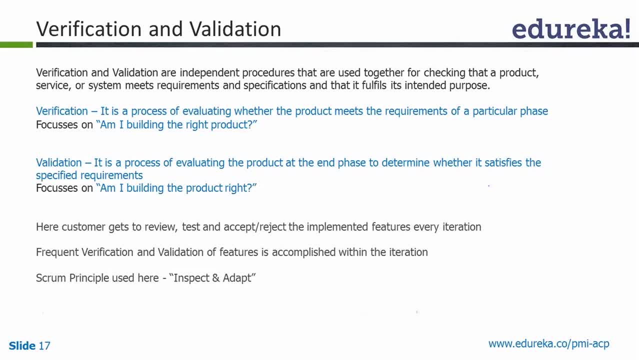 It's not actually the dynamic testing. It comes under the static testing, wherein you are following all the right kind of processes, And so that's as I said, it's more like a preventive Validation. is the actual testing? Okay, Okay. 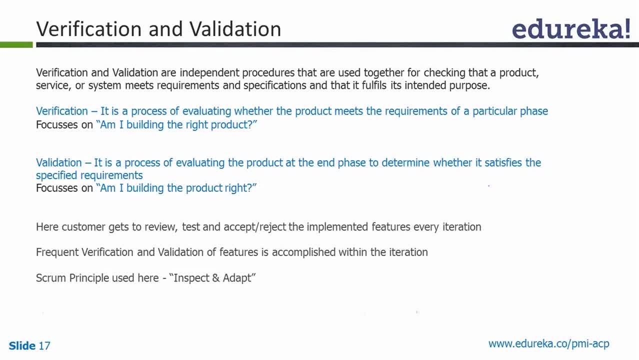 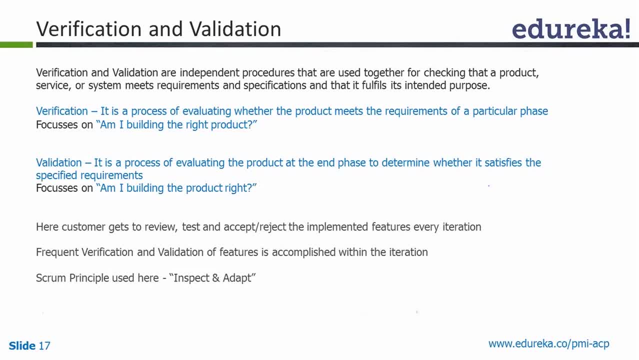 Right, So and okay. can you relate it to Agile now? Yeah, So acceptance, TDD is it's more like, It's more like making the verification strong. So VNV, I mean, I'm not looking for it's interlinkage from a TDD, TDD or APD perspective. 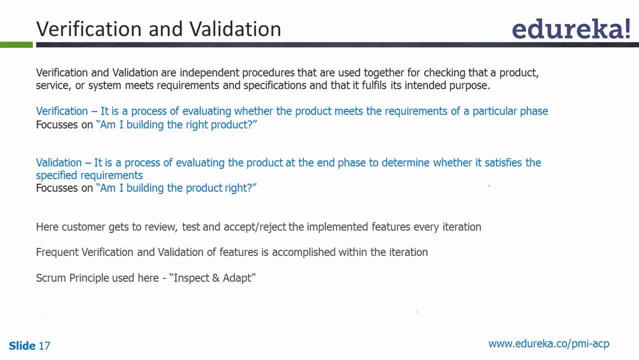 but in general, whole Agile, Agile method, Agile method. Okay, Thank you. Thank you. Verification is the unit. testing is an example of verification. it's done by the developer in a stage and the validation is done by the testing team once the feature is complete. 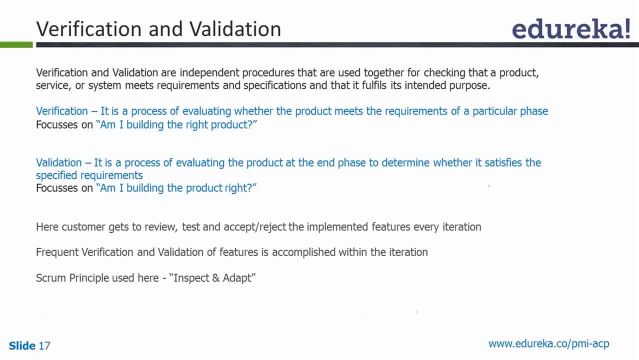 So correct. but validation, verification and validation is inspect and adapt. In verification you say: am I building the product right, while in Agile, when you are inspecting, you are checking: are we doing something right, right and validation is something. then you are saying: am I building the correct product? and then here we are saying, in, adapting once.